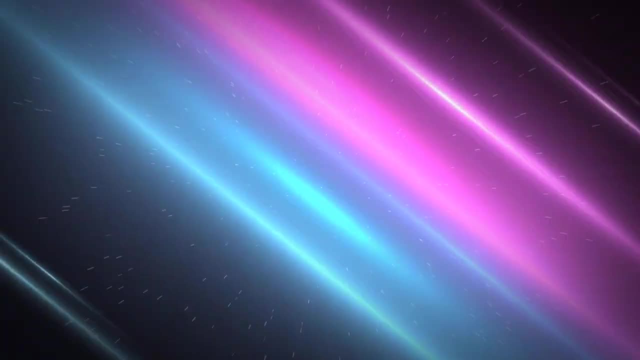 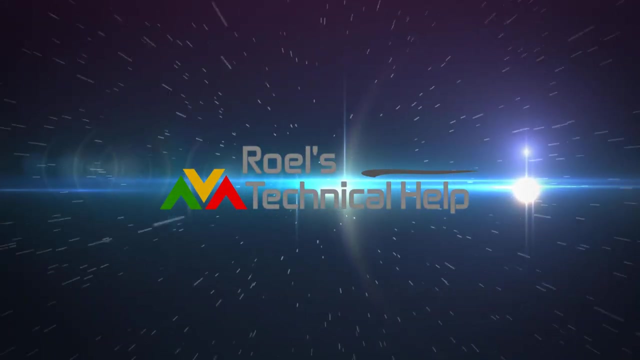 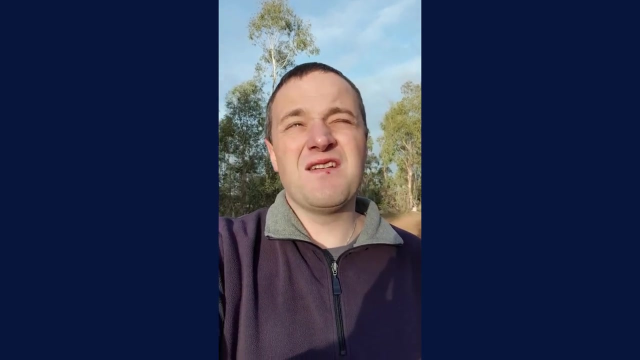 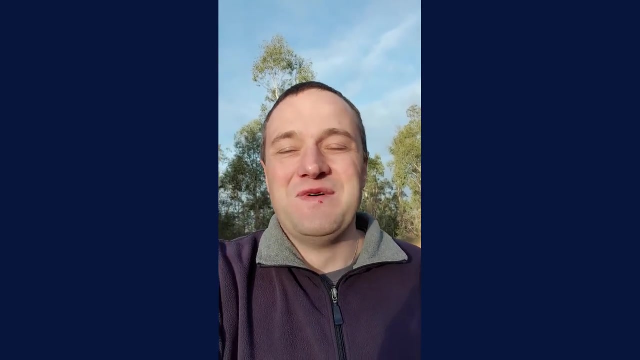 Morning YouTube. it's morning here. It might be like 1am at your place and you're trying to get out of the office. What are you doing in the office at 1am? Anyway, you might have a technical issue and this video will show you the question. 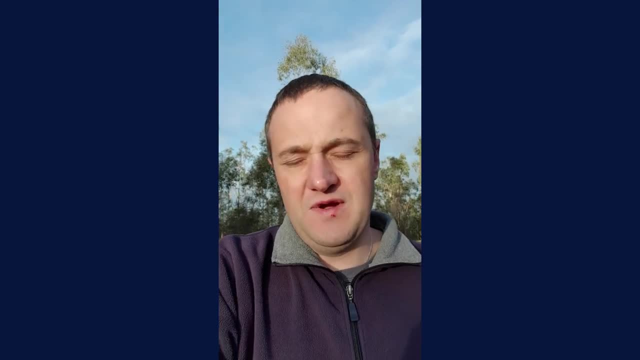 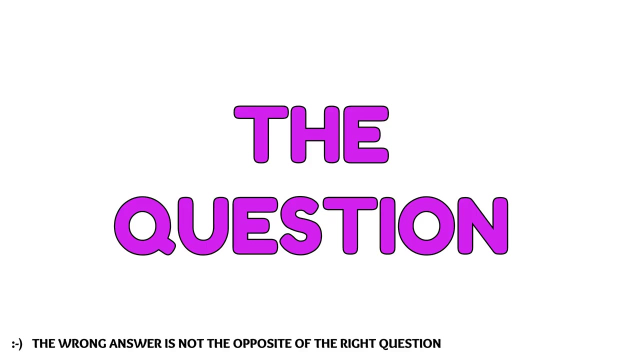 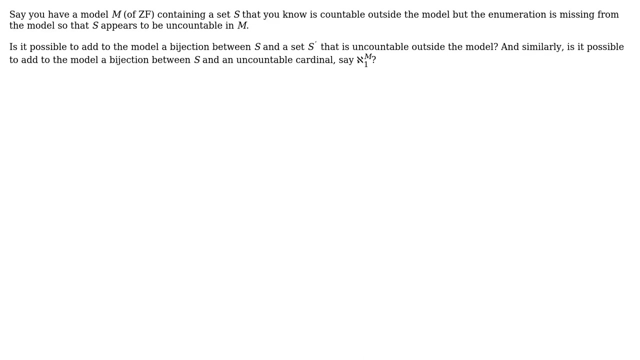 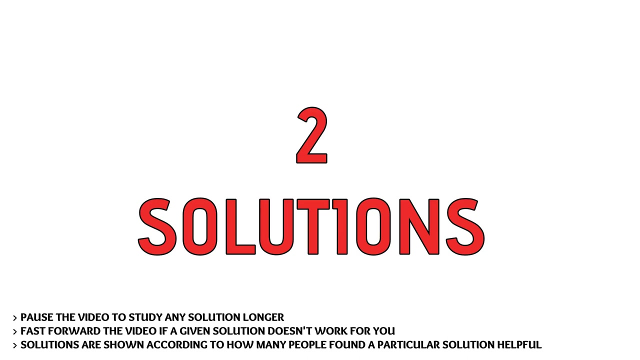 As well as the possible solutions. Hope you like it. Hope you subscribe to my channel- That will really help me and my family. And also that you like the video. Thank you, God bless. I hope you enjoy watching my video. I'm sorry I can't share it with you guys. 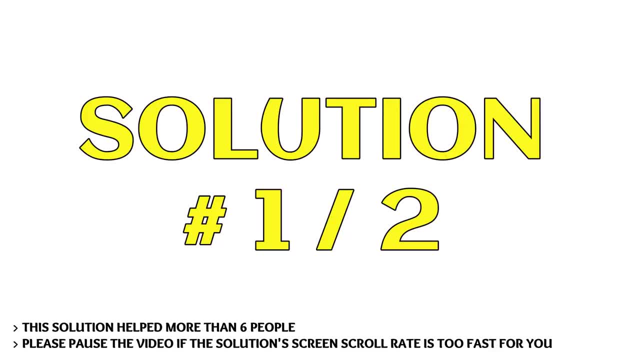 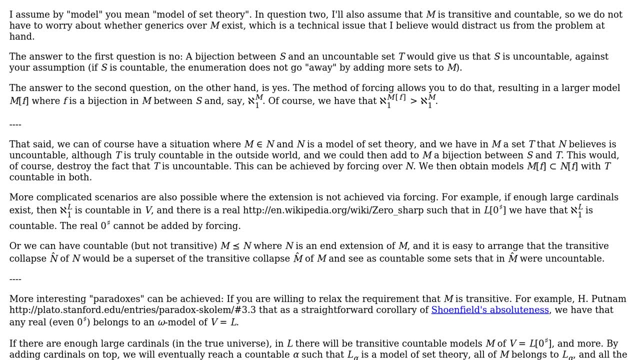 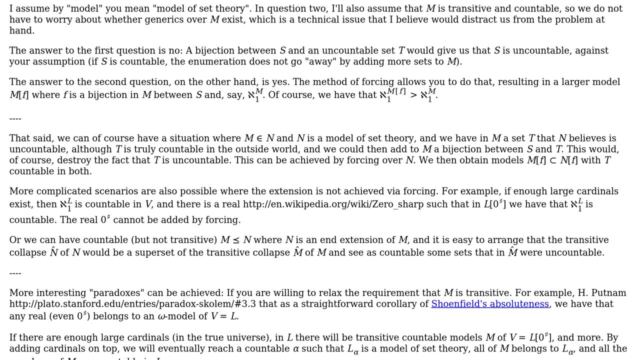 I hope you have a good day. I'll see you later. I'm sorry I left the video. Sorry. Next video is gonna be the previous video. I will post the winner. So before that, bye, bye, Goodbye, Take care. 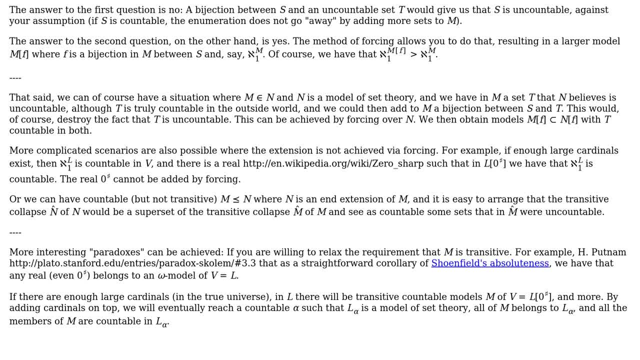 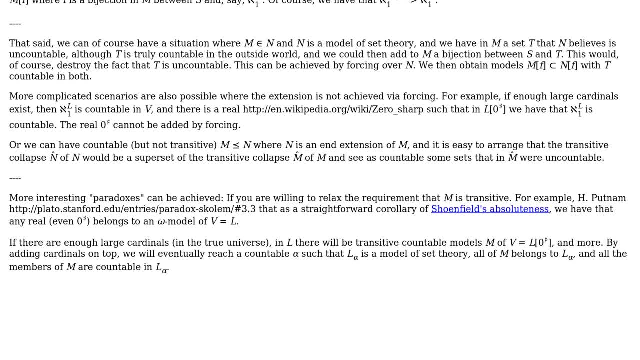 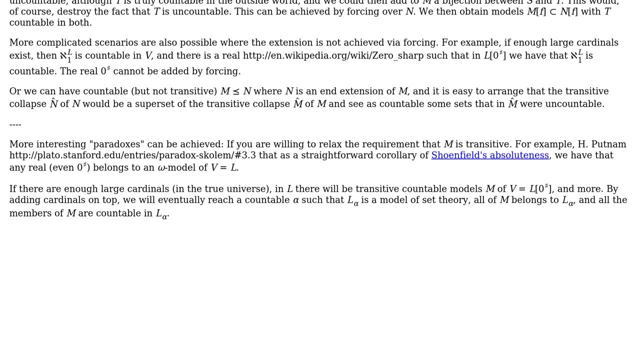 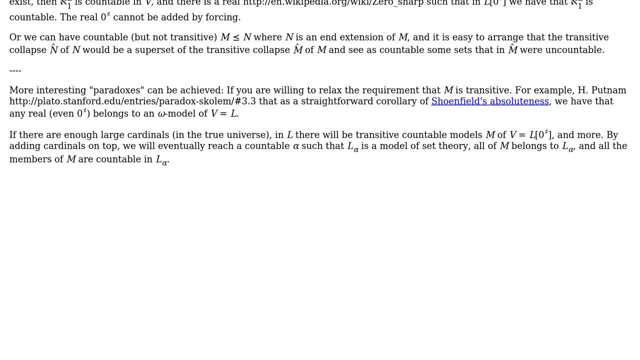 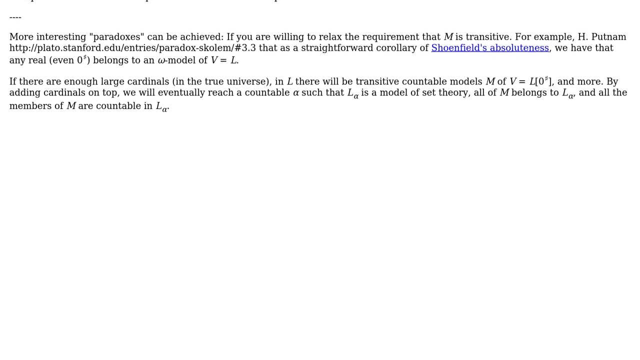 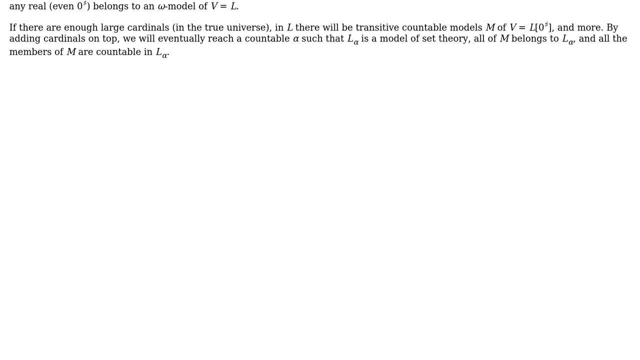 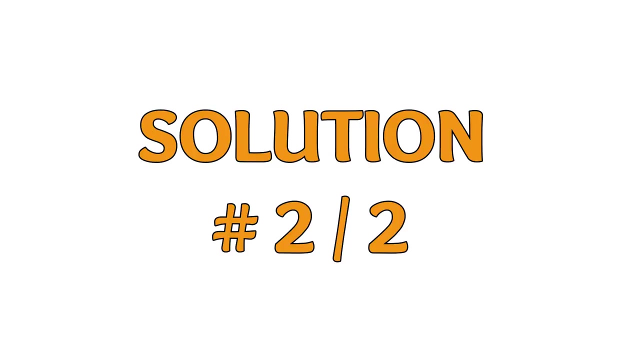 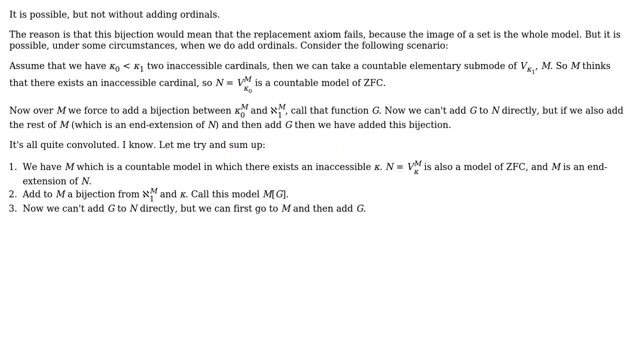 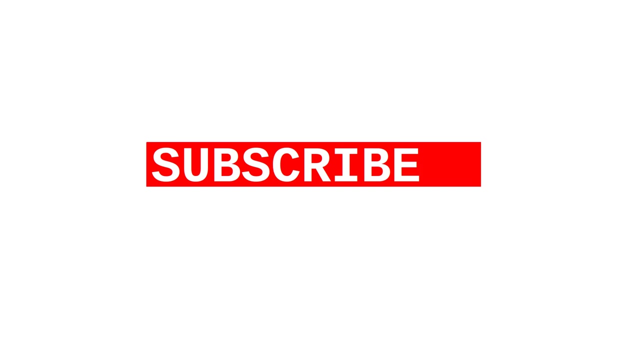 Bye, bye, Bye, bye, Bye, bye. Thank you, Thank you, Thank you, God bless.